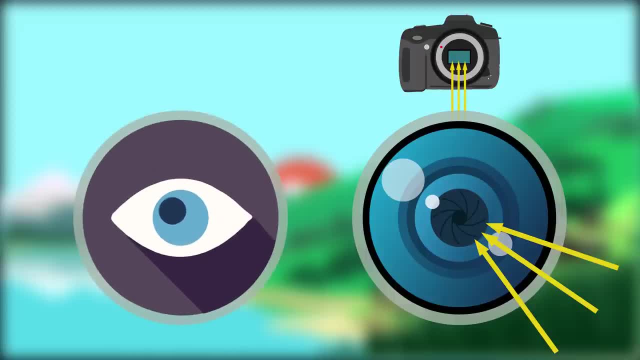 camera sensor. To understand, let's look at the human eye. All cameras are designed like human eyes. The cornea of our eye is similar to the front element of the lens, gathering light and bending it inward toward the iris. The iris can expand or shrink, controlling the size of the 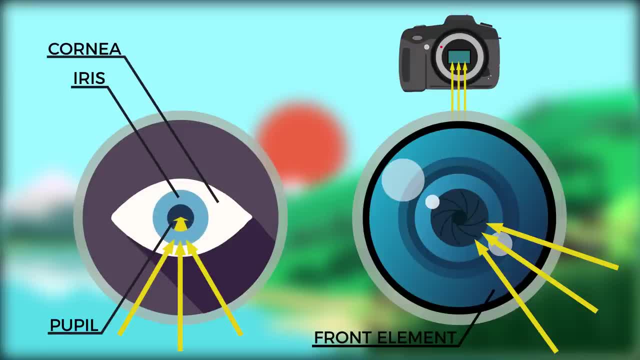 pupil which passes light into the inner eye. The pupil is what we refer to as the aperture in photography. The amount of light that falls onto the retina is determined by the size of the pupil. The larger the pupil, the more light falls onto the retina, The larger the aperture. 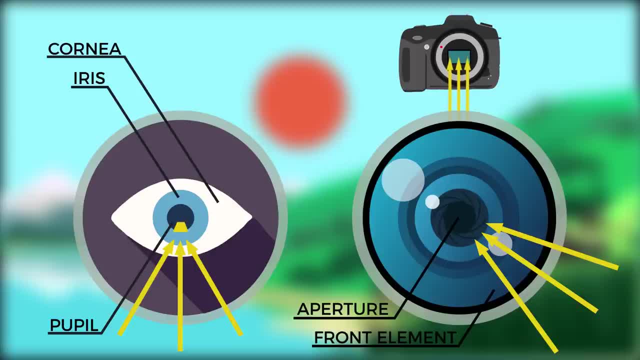 of the lens, the more light enters the camera. The iris of the lens controls the size of the aperture and is called the diaphragm. The diaphragm's function is to block all light, with the exception of the light that goes through. 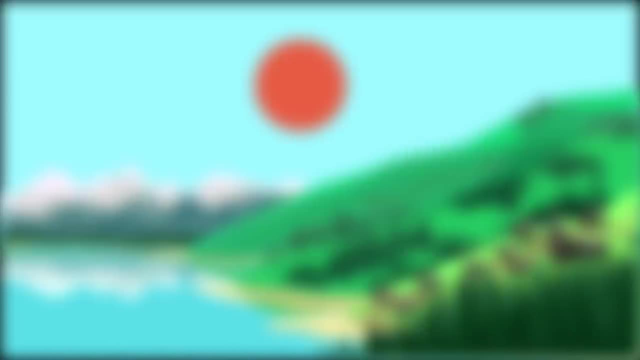 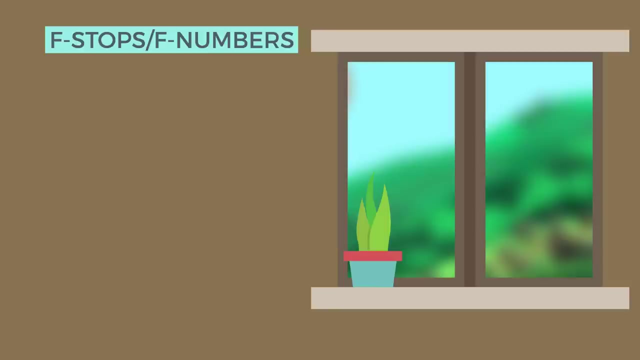 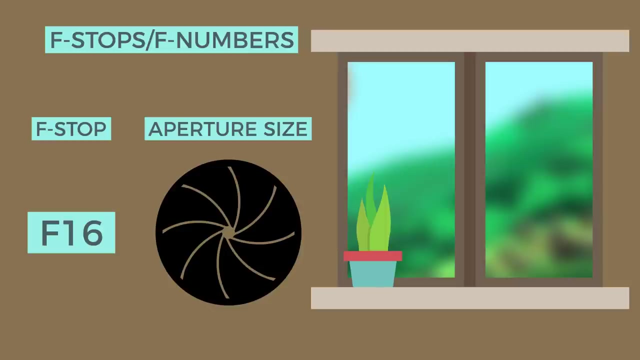 the aperture. In photography, aperture is expressed in f-numbers, also known as f-stops. F-stops are a way of describing how open or closed the aperture is. The smaller the f-stop means a larger aperture, while a larger f-stop means a smaller aperture. This can be tricky. 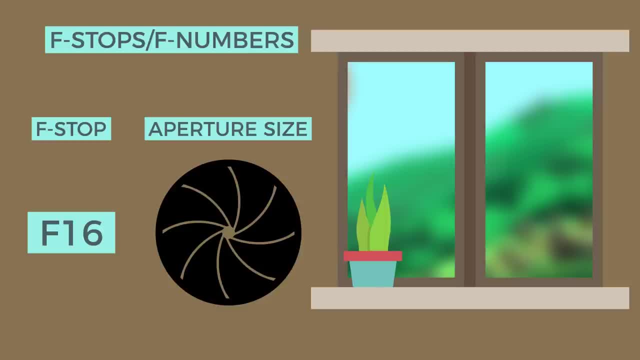 to remember, since large f-stops mean small aperture sizes. So an f-stop of f-1.4 is larger than f-2.8, and much larger than f-8 or f-11.. Aside from controlling the amount of light passing through the lens and into the camera, 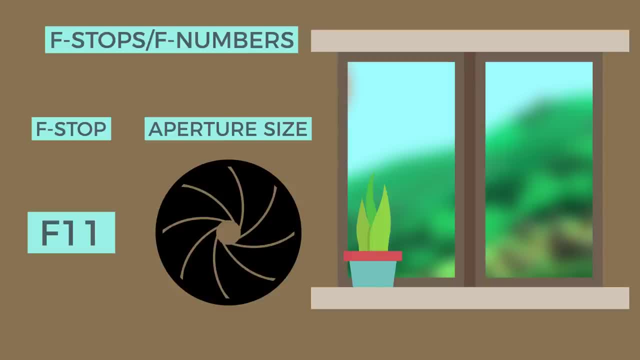 the aperture has a direct impact on the depth of field, the area of the image that appears sharp. A large f-number, such as f-16,, will bring all foreground and background objects into focus, while a small f-number, such as f-1.4, will isolate either the foreground, 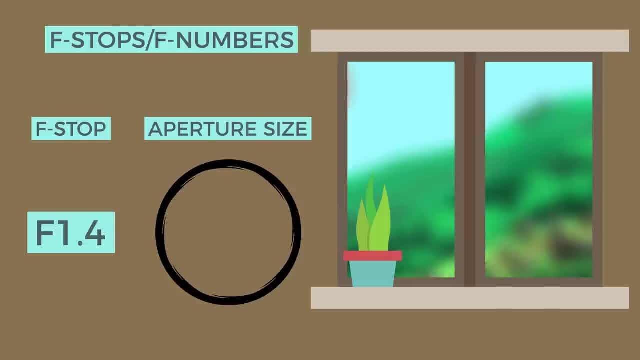 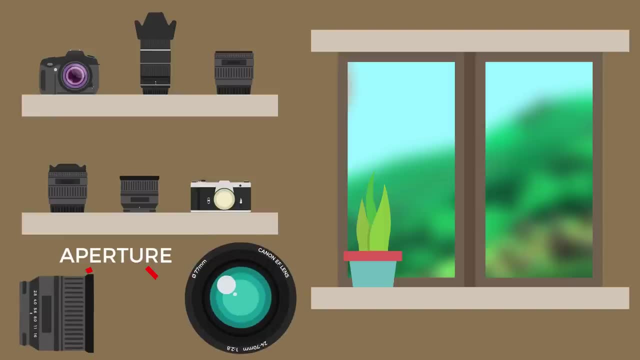 objects and make everything else blurry. Every lens has a limit on how large or small the aperture can get. If you take a look at the specifications of your lens, it should indicate the maximum apertures and minimum apertures. The maximum aperture of the lens is much more important than the minimum aperture because 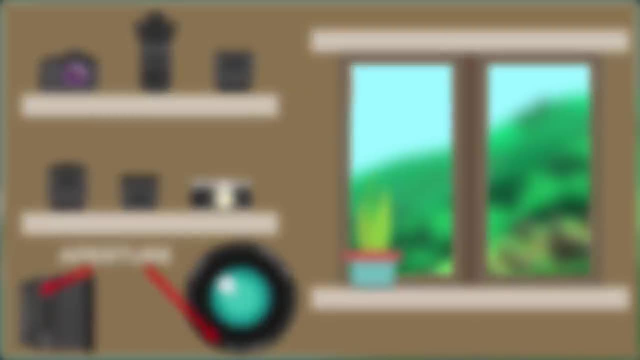 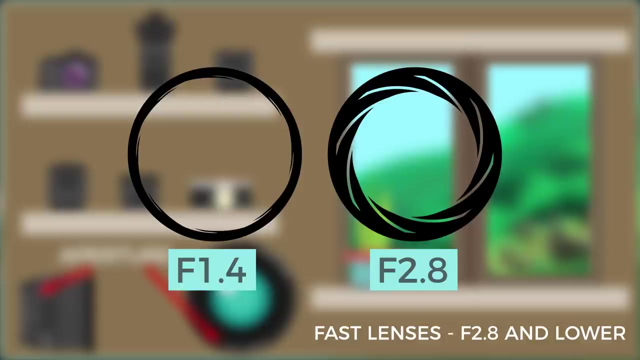 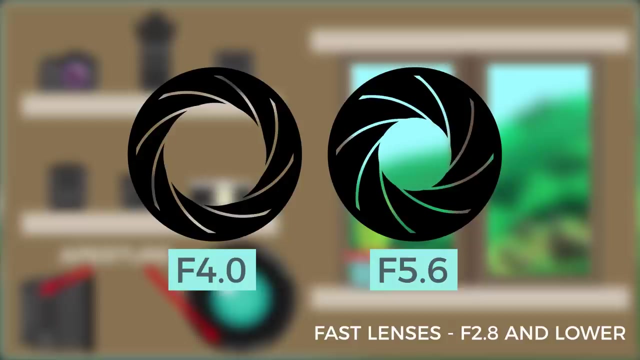 it shows the speed of the lens. Lenses with apertures of f-1.4 or f-2.8 are considered fast lenses Because they can pass more light into the camera than, for example, a lens with a maximum aperture of f-4 or f-5.6.. That's the reason night photography usually requires fast lenses. 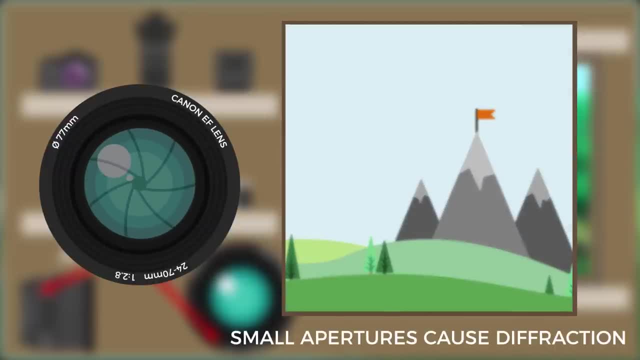 The minimum aperture of a lens is usually not important and should rarely be used, as diffraction will cause the image to lose clarity. It is also worth noting the two types of lenses: primes and zooms. Prime lenses have a fixed focal length, meaning they cannot zoom without. 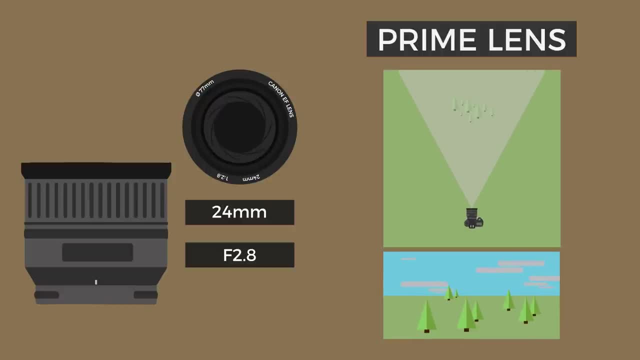 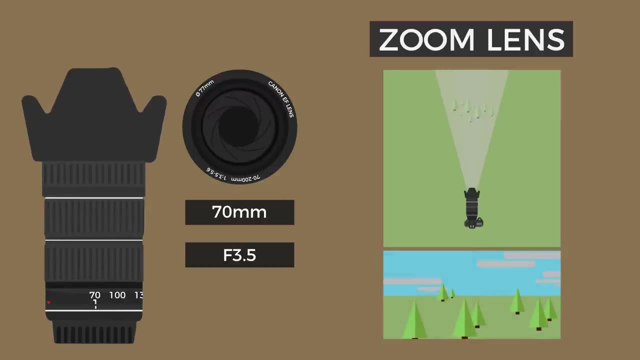 physically moving closer or further away from the camera. This means that the focal length is either longer or further away from the subject. Zoom lenses give you the flexibility for you to zoom in or out of an object while remaining stationary, While prime lenses will have a fixed maximum aperture- the maximum aperture of a zoom lens. 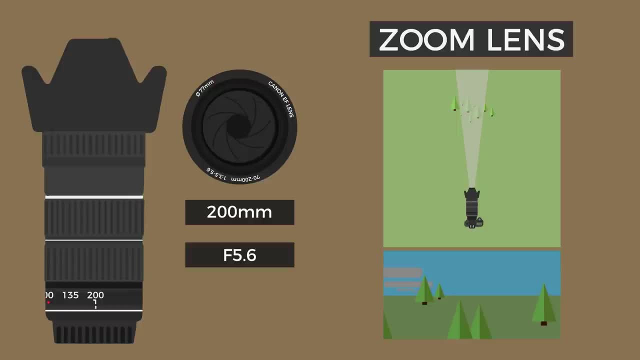 will often get smaller as the focal length increases. These lenses are called Variable Aperture Lenses. This is important because for a zoom lens with a focal length of 70-200mm, the aperture may increase from f-3.5 to f-5.6.. The aperture may also be reduced to a maximum aperture of 1.8.. This means that the aperture increases from 1.8 to 1.8.. The aperture increases from 1.8 to 1.8.. The aperture may also increase. 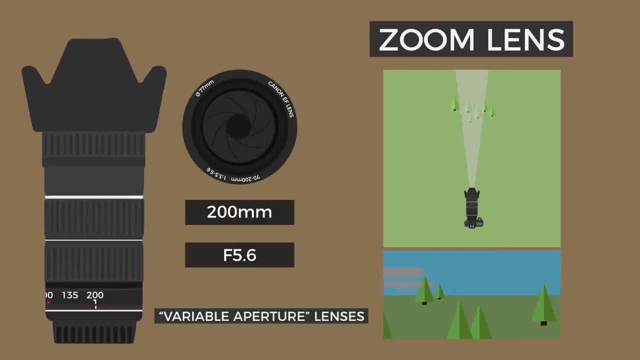 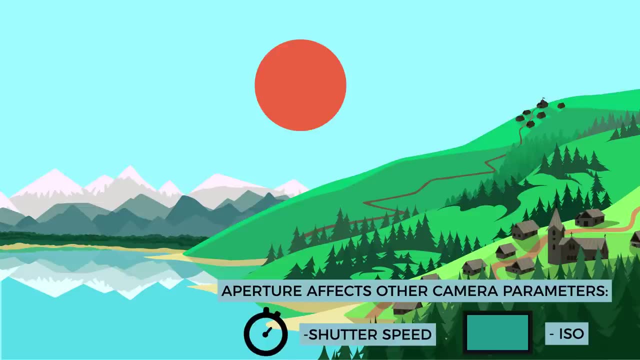 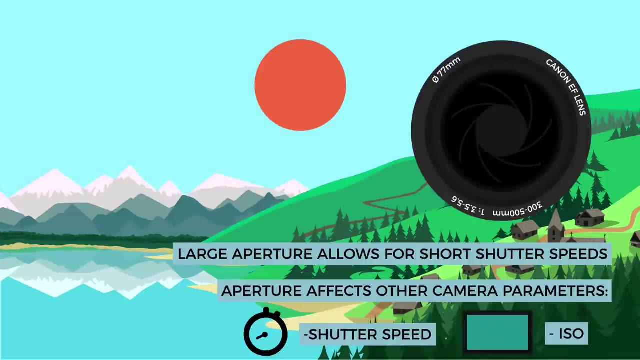 decreasing the amount of light entering the camera. Because aperture controls the amount of light entering the camera. it also affects other parameters such as ISO and shutter speed. A larger aperture or smaller f-number will let more light into the camera, allowing you to use a faster shutter speed or lower ISO value. 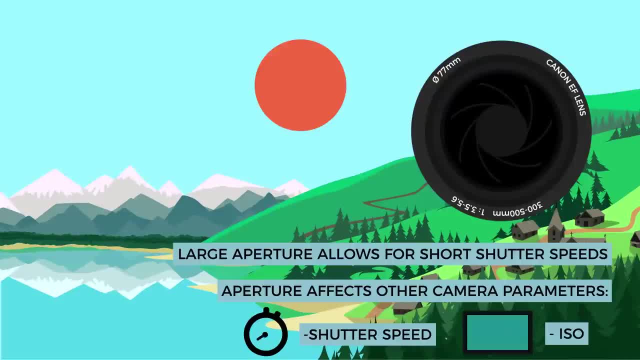 This is beneficial to eliminate motion blur and reduce the amount of noise that your camera will produce if its ISO gets bumped up Faster. shutter speeds can be essential in scenes with lots of motion, like sports and wildlife photography, So a fast lens can help increase your shutter speed. 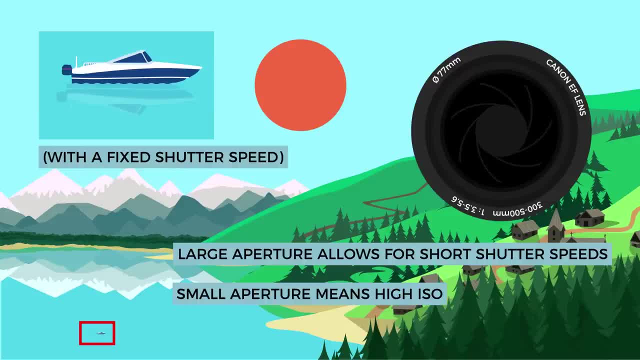 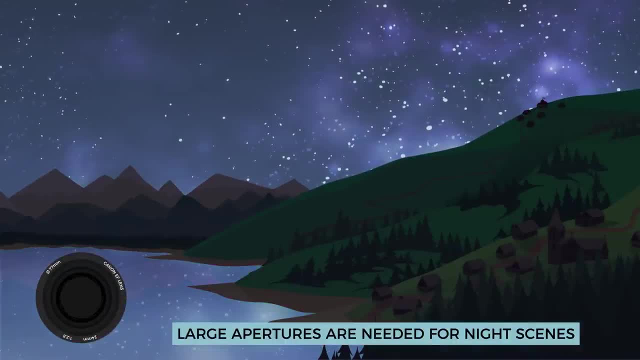 or decrease your ISO value if your shutter speed is set to a specific value. Fast lenses are also imperative for any kind of nighttime photography. Whether you're taking pictures of the Milky Way or doing a moonlit photoshoot, large apertures will let as much light in as possible. 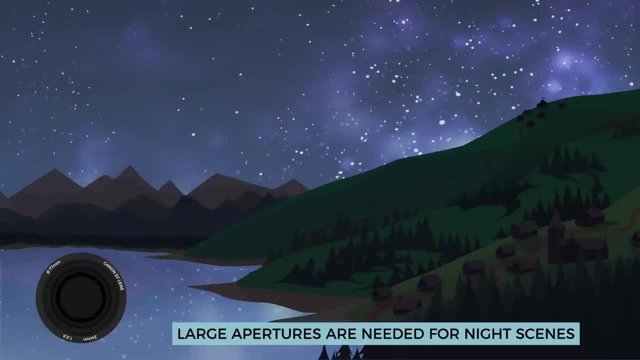 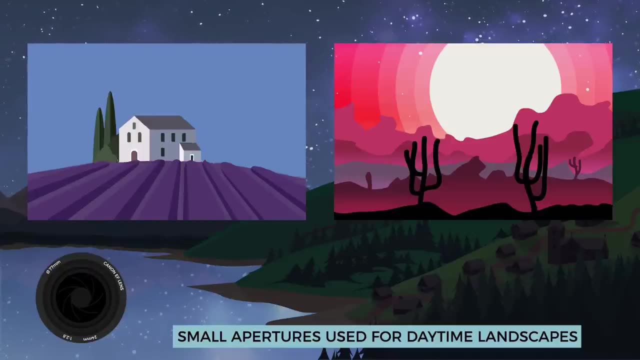 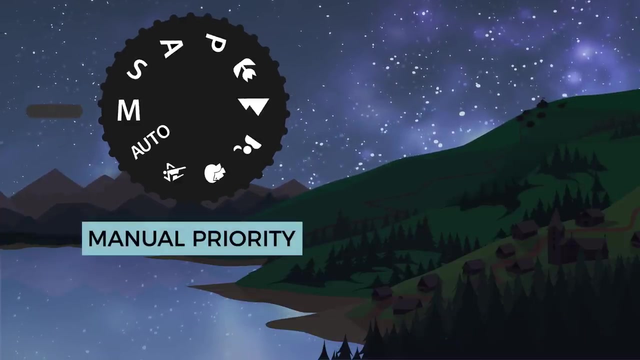 Small apertures can be useful as well. Shooting landscape scenes requires everything in crisp focus, so smaller apertures will sharpen any out-of-focus areas that may come about. To enable manual adjustment of aperture values, set your camera to either aperture priority or manual mode.